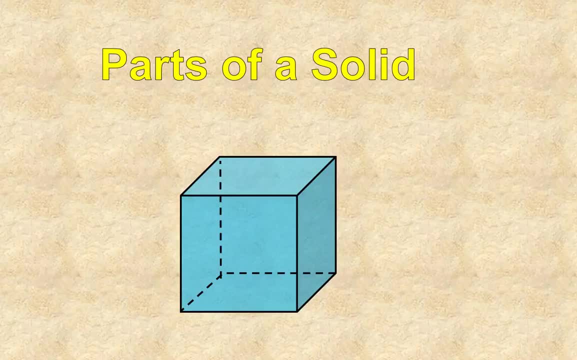 points meeting together in a vertex. So let's go ahead and count the vertices. That, by the way, vertices is the plural form of a vertex, So we're going to count the number of vertices in this solid. There's one here, another down here, three, then four, five, six, seven and eight. 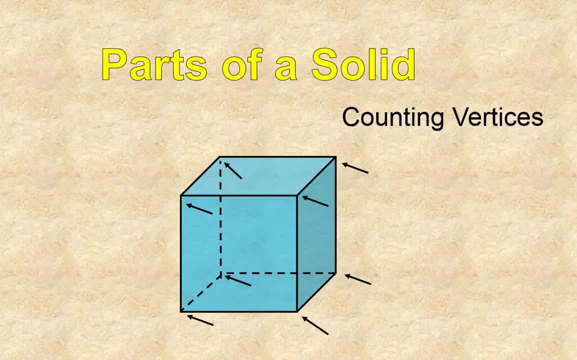 Notice that there's three vertices. Sometimes they're called corners, but the correct math term for it is a vertice or, in singular form, a vertex. All right, Another part of a solid is an edge. On a two-dimensional polygon, for example, you would: 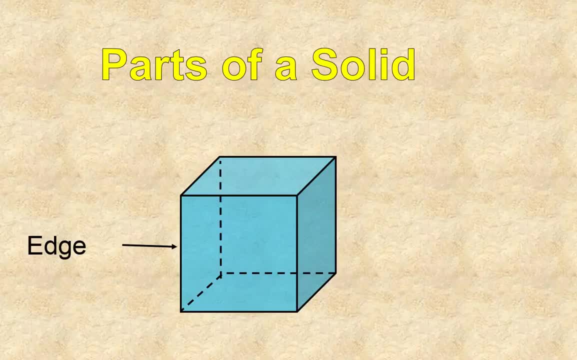 have a side. Well, with three dimensions, you have an edge and you can see that there's an edge there where two. well, I don't want to get too far ahead, so let's just go ahead and count the edges. 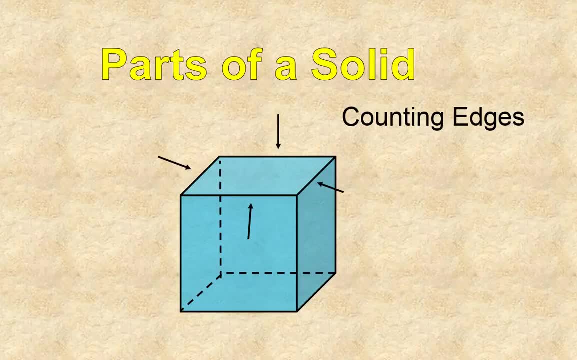 There's one, two, three, four edges on the top of this solid. one, two, three, four edges on the bottom of this solid, and then we can't forget those upright edges there, there, there and there. So we have four on the top four. on the bottom four, around the edge, There are 12 edges. 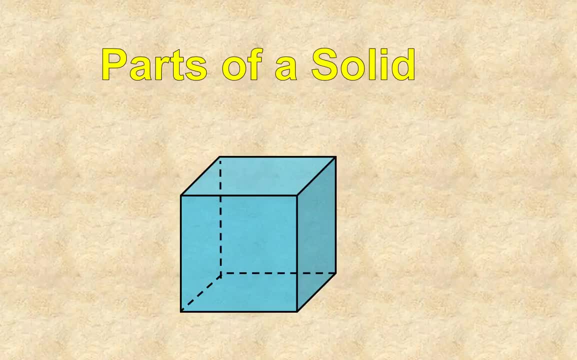 in this solid. The final part of a solid is a face. That's that vocab word I just about said when I was saying where two faces meet they create an edge. But a face like this is a solid flat surface or the flat surface of a solid. So we're going to count the number of faces we have here. We have one, two, three, four, five and six. All right, There are six faces of this solid. 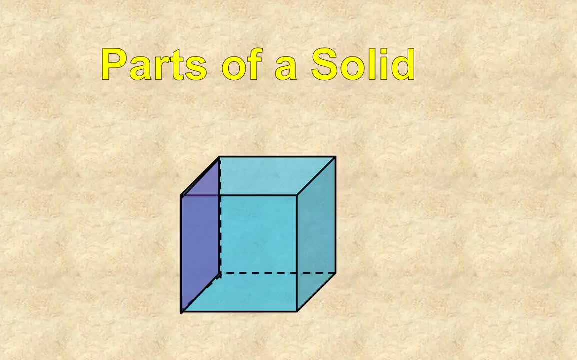 Now, if you recognize this, maybe, and said: hey, I recognize that it it has. it looks like a die when I'm rolling a die And you know that it has six, six sides, or what we call sides, when you're rolling a die. 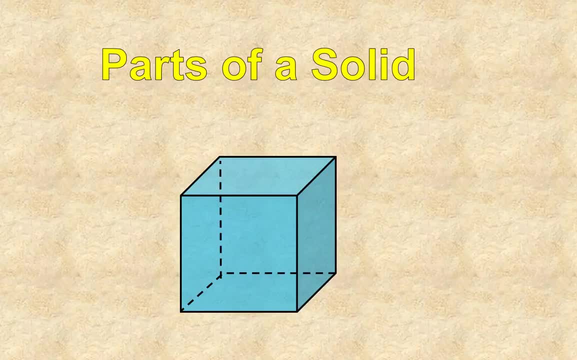 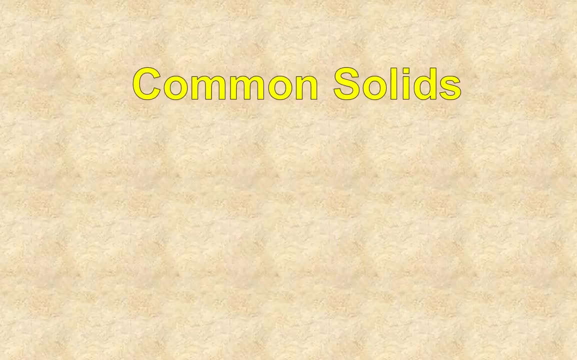 but it's six faces, Then you might have already known that, But it's important to be able to identify all the different faces, edges and vertices of a solid. Let's talk about a couple of common solids: The, the one that we were just looking at. 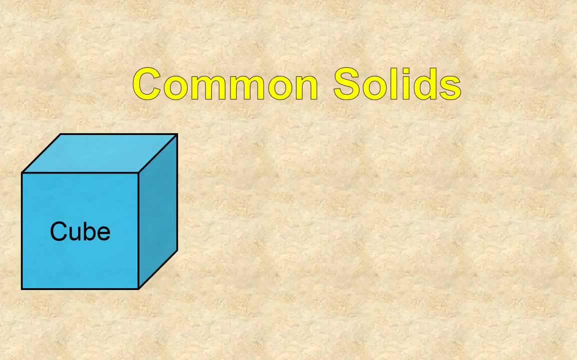 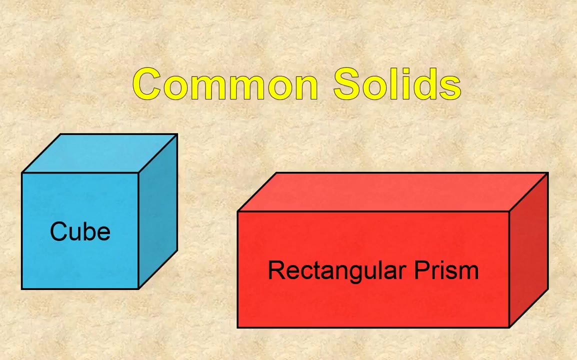 that's called a cube. A cube is a solid where each face is a square. So you have six squares that meet together at the edges and they form a three-dimensional cube. Another common solid is a rectangular prism. A rectangular prism is similar to a cube. only four of the faces at least are rectangles, Sometimes all. 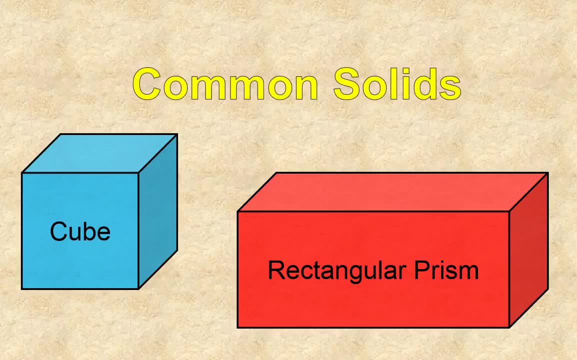 six will be rectangles, but at least four of them are rectangles. In this case, the, the face that is closest to us. the top, the back and the bottom are all rectangles. It appears as though the the sides are squares, but we would call this. 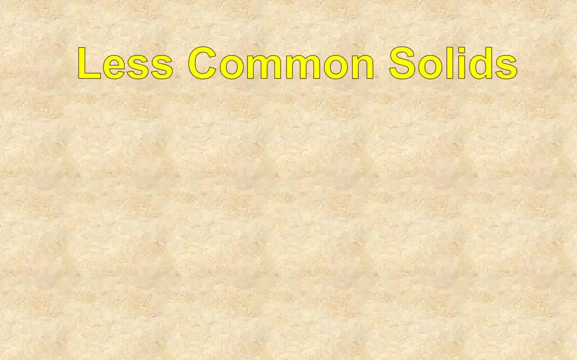 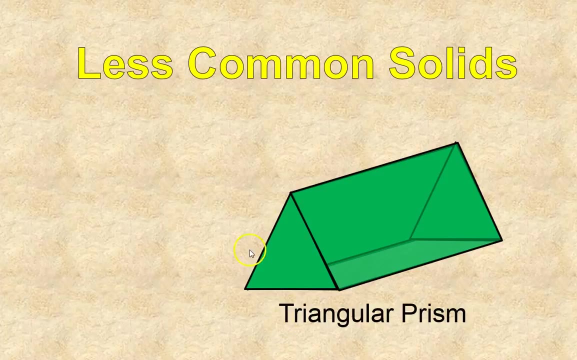 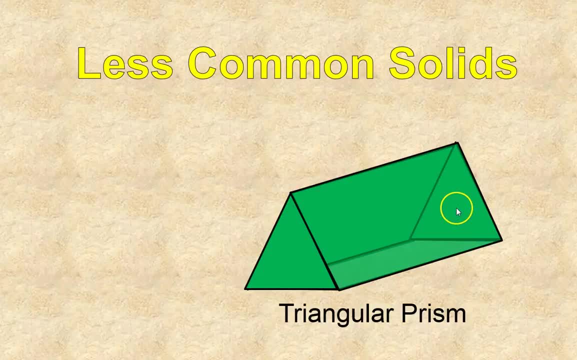 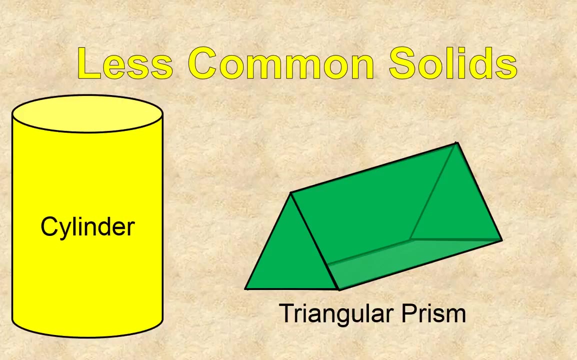 And these edges are faces here that are triangular- would be called the bases of this triangular prism, even though they're not on the bottom. So that's a try. they have triangular bases. that means it's a triangular prism and a prism that has a circle on the top and on the bottom, or in other words this: the 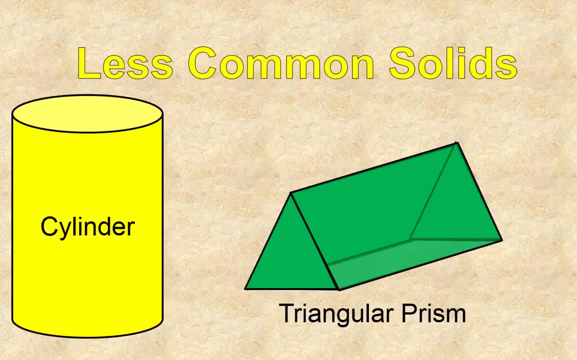 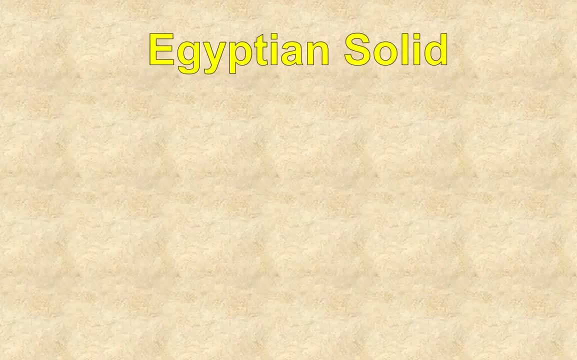 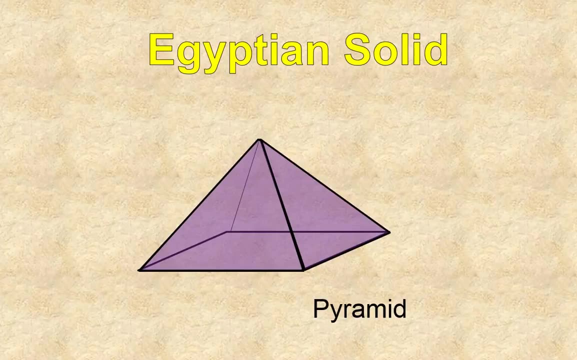 base is a circle, is called a cylinder. Alright, looks kind of like a tin. can We have our cylinder and our triangular prism? I want to talk about one more solid, the Egyptian solid known as a pyramid. A pyramid has a base of different form, different polygons. This one here has a 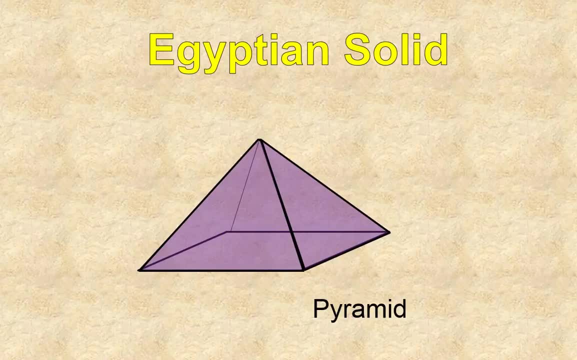 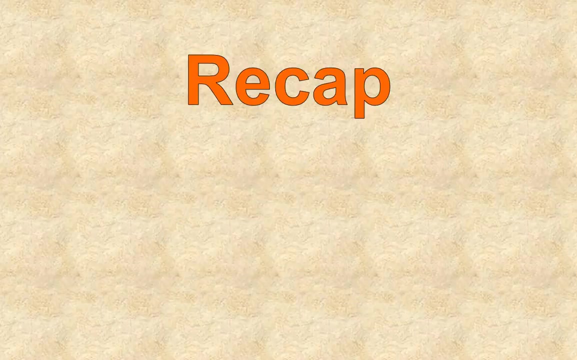 square as our base and then triangles meeting up at a point. You can also have a triangular pyramid where the base would be a triangle and those points would come up to meet here at this vertex where you have those faces Kind of leaning in to meet at one common vertex up top. So that's a pyramid, Just a.